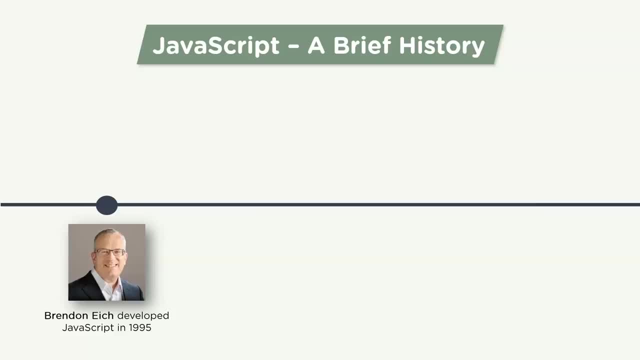 at Netscape at the time and was implementing Java, the hot buzzword for the browser. Later he developed a more easy-to-use programming language called Mocha. The idea was to make Java available for big professional component writers, while Mocha would be used for small. 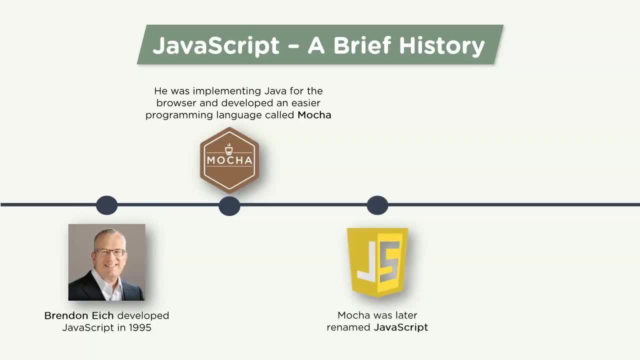 scripting tasks. Mocha was later renamed to JavaScript. Now, in 2009,, Nodejs was released. This allowed programmers to write full applications in JavaScript. NPM was also created for installing reusable bits of code in libraries. So, moving on, what exactly is JavaScript? 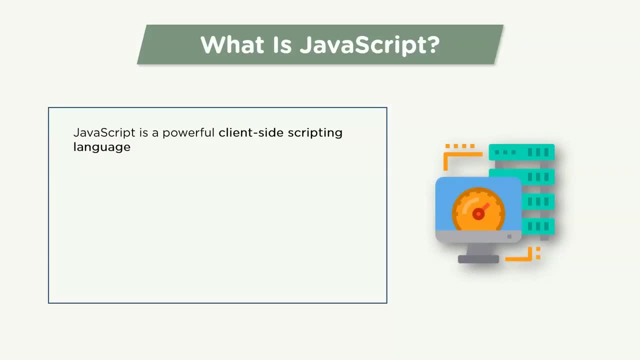 JavaScript is a server-side and client-side programming language. It is commonly used to create web applications. Now, all of these applications in JavaScript can be seen in diverse fields like gaming, web development, server development, robotics, among others. Popular JavaScript libraries and frameworks like ReactJS and Angular have scaled tremendously. 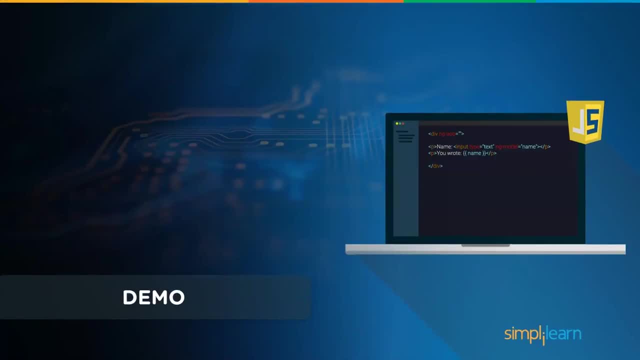 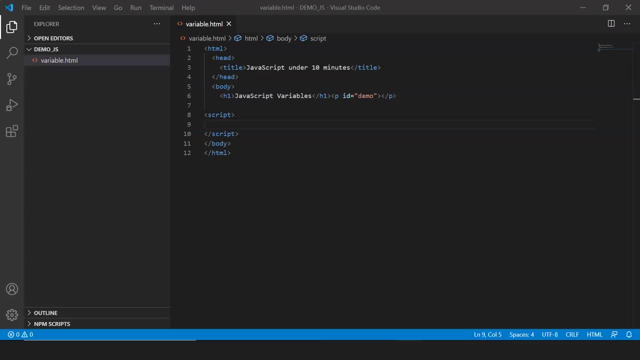 in the past few years. Moving ahead, let me show you a simple demo to implement a few concepts of JavaScript. Let's head to VS Code for this, Alright, so back in my VS Code, I've created a folder called demo- underscore js. within. 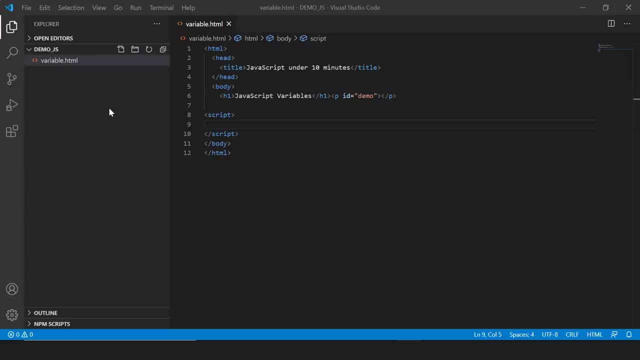 which I've created a file for variables, which is the HTML file. Alright, I've also added the initial code for it, with the title tag and the heading tag, And now, within the script, I'm going to define my variables. So here let me say var, the keyword var, and say x. 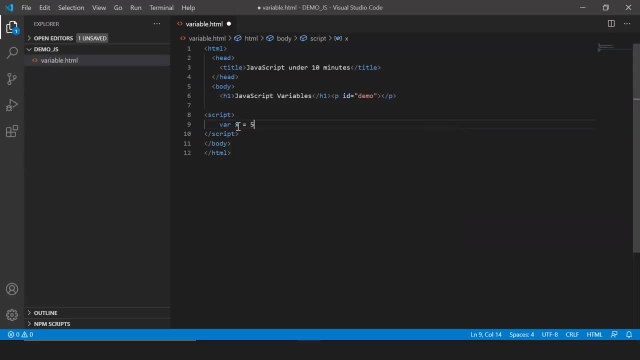 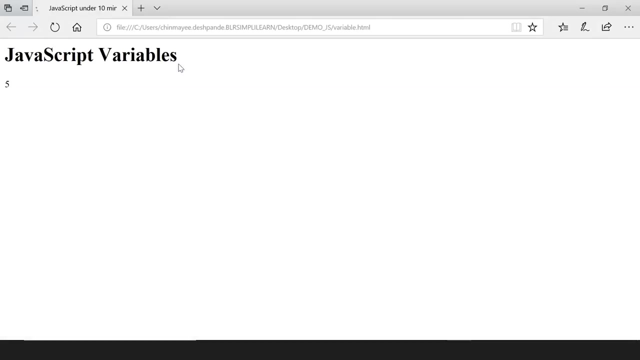 equals 5.. Now JavaScript is loosely typed and also all these variables can be declared as and when they're being used. Alright, so with this variable I can just print it out. Let me say: document dot, write x. Alright, so let's go and open the file. Alright, so here you. 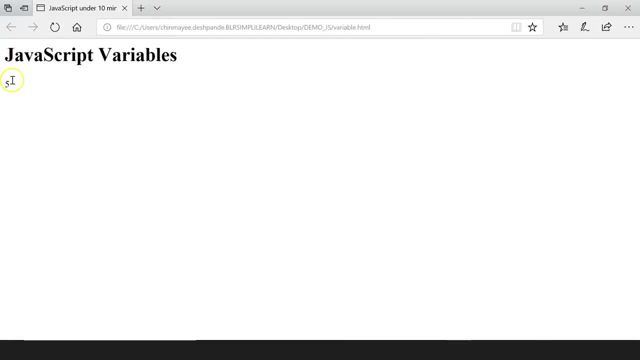 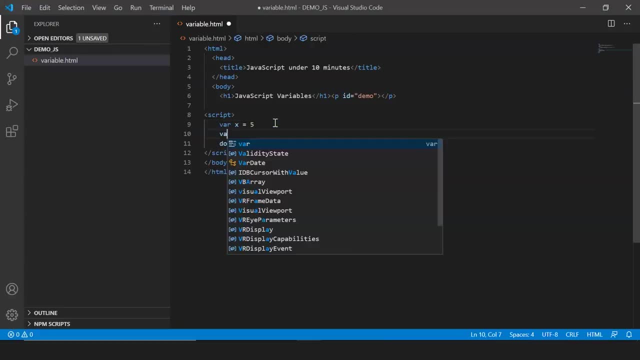 can see, the heading has been displayed with the value of x, that is 5.. Now we can also perform various actions on these variables. So let me say: variable y equals 3.. And then let's say: variable sum equals x plus y. And here let me just output the. 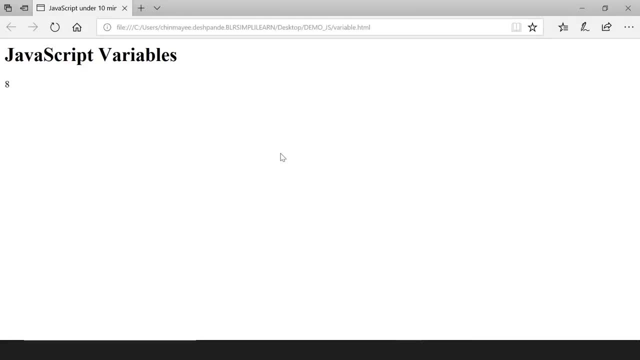 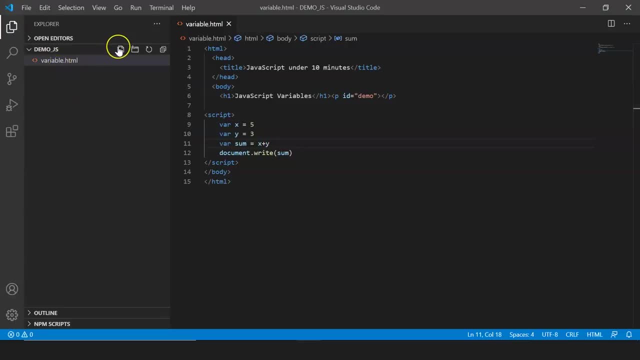 sum. Let's have a look at the browser It displays: 8.. Alright, So now let's go ahead and create another HTML file to understand how arrays work in JavaScript. So let's say: arrays, welcome javascript. So let's say: arrays, welcome javascript. 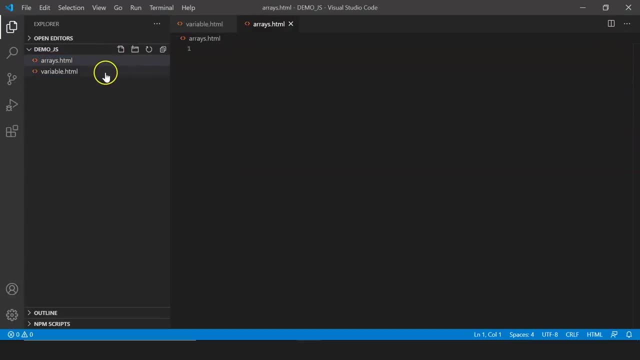 Let's open JavaScript dot HTML. all right, let me just copy the initial code for the same. all right, I've added the initial code for it and now let's go ahead and create an array. so here let me say let I'm going to create an array of cars, so let's say cars within. 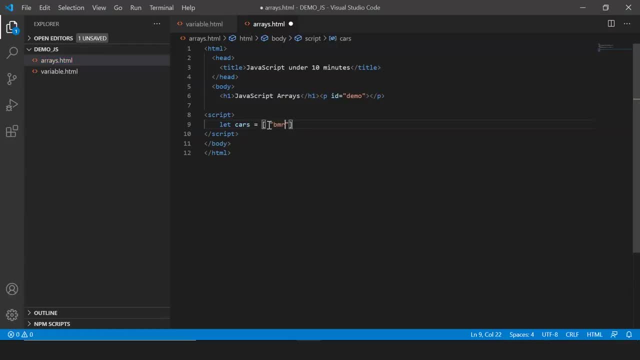 which I say BMW and then I say Volvo and then I say Honda. all right, so we successfully created an array. now we can just output it using console log. say console log cars of 0, which indicates the value of the array at the position index at the end of the array. so let's say console log cars of 0, which indicates the value of the array at the position index at the 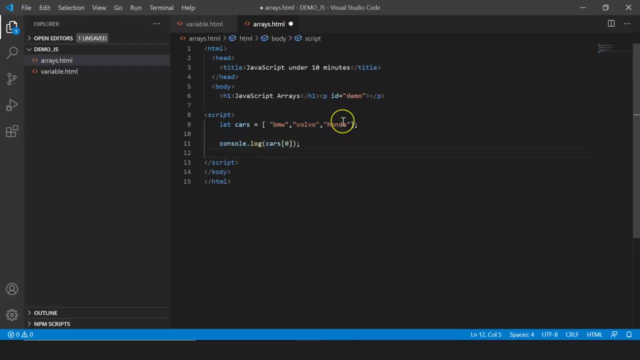 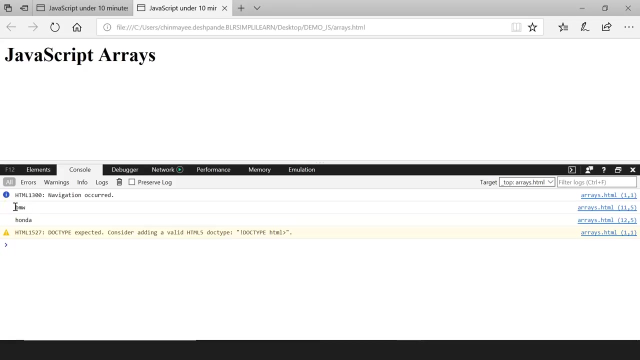 index position 0. similarly, let's just say console dot log, cars 2: all right. so when we save it and then execute it, let's see, let's have a look at the browser, you can see it's displayed BMW, which was at the index position 0, and 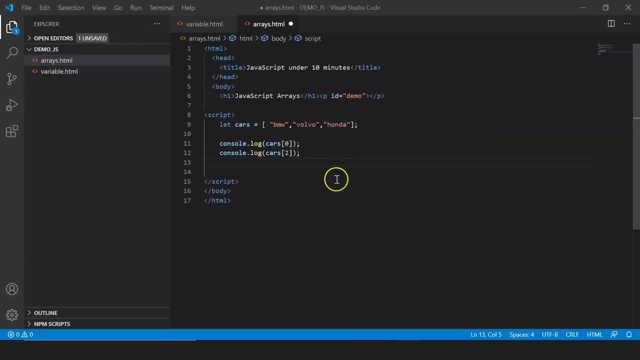 then it's displayed Honda, which was at the index position too. now let's display the length of the arrays. so for that we can make use of the length from here property and say carslength here and after this we'll just consolelog it. So let's say length. 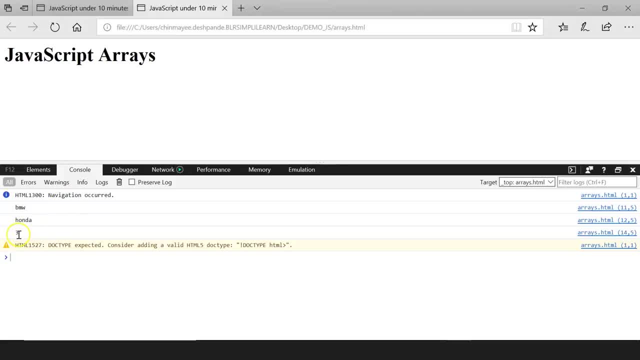 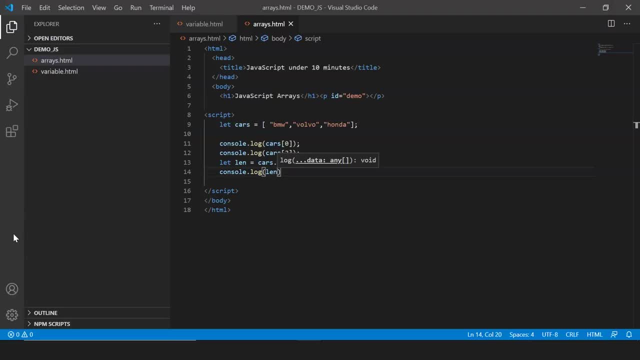 So when we have a look at the browser, we have 3 here which indicates the length of our array. Now we can also perform other actions, like looping over it. So let's have a look at JavaScript loops. So I'm going to create another file here and say loopshtml. 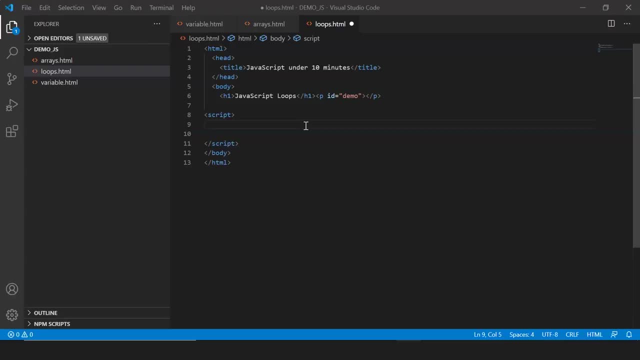 So I've also added the initial code now. So now let's first look at the simple for loop. So here let me say: let me create a variable called n, and then I'll say documentwrite, Let's display a simple message saying the number. 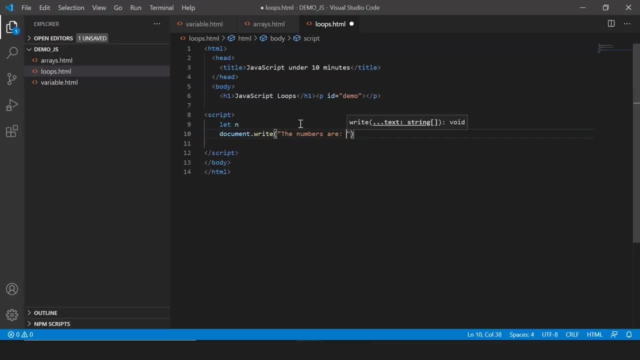 The numbers are and we just break the line Now to display the numbers from 0 to 9. I'm just going to use the for loop saying for n equals 0,, n less than 10, n++, and then I'm going to display the values. so I say documentwrite. 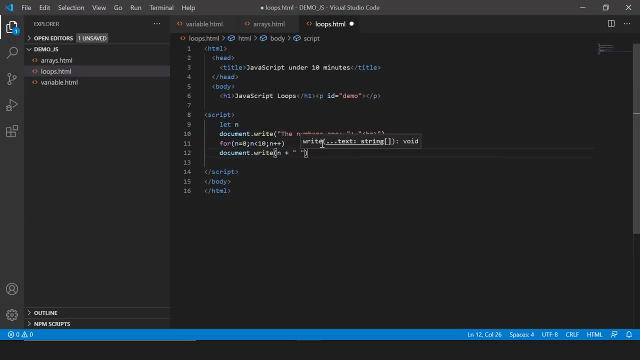 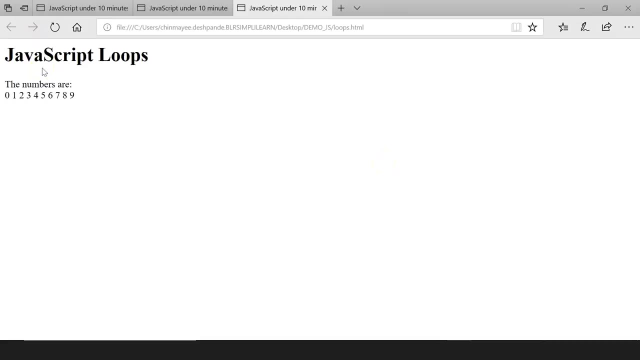 n. Let's just give a space between the numbers. So yeah, All right. So now when we have a look at the browser, you can see it says the numbers are and it displays the digits 0 to 9.. Now let's look at another example for loops. 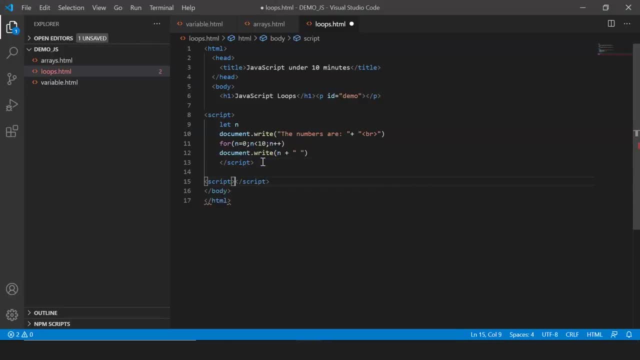 So I'm going to create another script tag. and now let me just say documentwrite. Now I'm just going to add space, add two lines from the previous one. So let me just add these first, all right. And now let's say let y equals. I'm going to create an array. 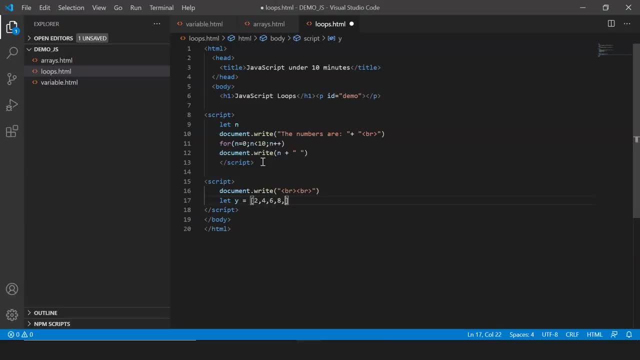 So let's say 2,, 4,, 6,, 8,, 10,, 12 and 14, yeah. and then let's say: for I'm going to create an index variable, that is i. i equals 0 to lent. 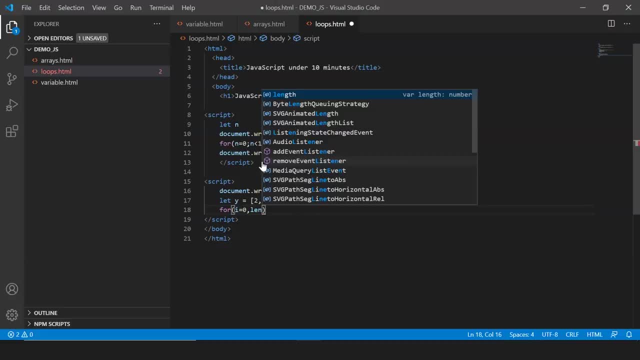 I'm going to create an index variable, that is i. i equals 0 to lent. I'm going to create an index variable, that is i. So let's say i Length equals ylent and sum equals 0, and i less than length, i++. 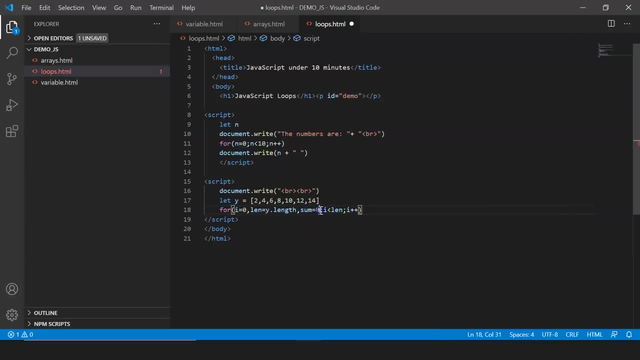 So here I've just created three different variables and initialized them here. So I've created an index variable i, a length variable for length, and then we have the sum variable that records the sum of the x, And then I've made sure that the variable i is less than the length. 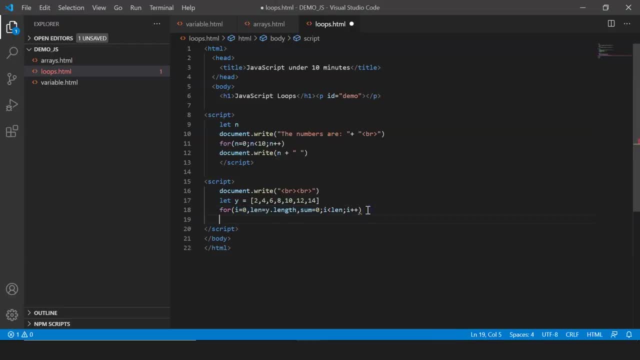 And then I've used the increment operator. So now let's say: sum plus equals y of i and then say documentwrite: the sum is sum, all right. All right, Let's save and execute this. So here you can see that the sum 56 is being displayed. 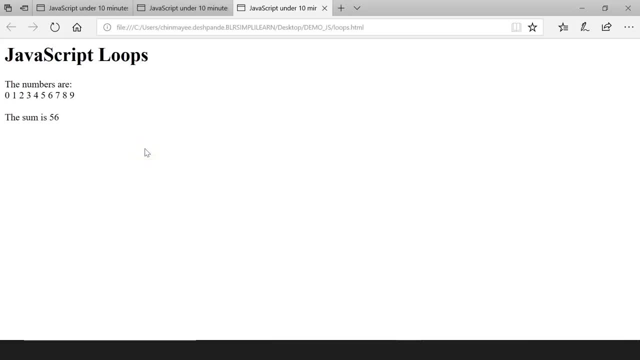 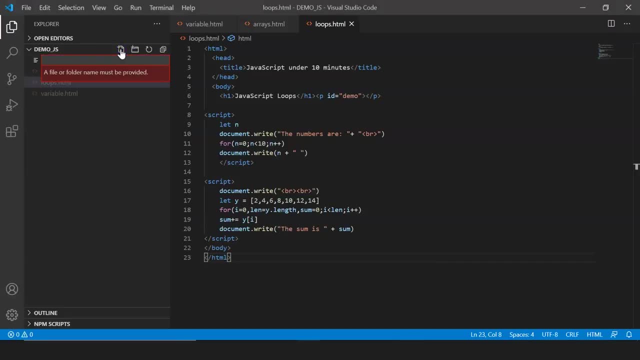 So this is how you make use of loops. You can also use the while loop. However, I'm not going to get into the details of it. I'm going to help you understand how functions in JavaScript work. So I'll say functionshtml, and let me also add the initial code. 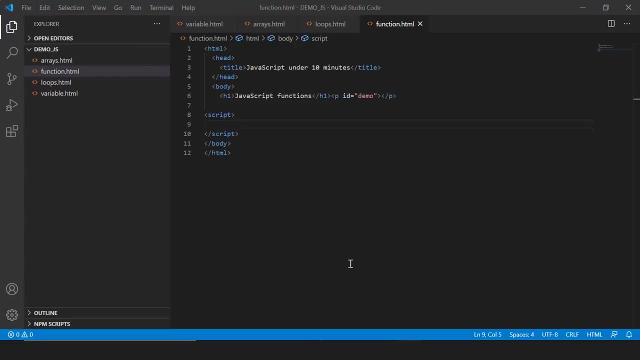 All right. So now. one thing to remember is that there are various ways to define a function in JavaScript. However, in this video, I'm going to show you two different methods. One is using the function constructor and the other one is using functions expressions. 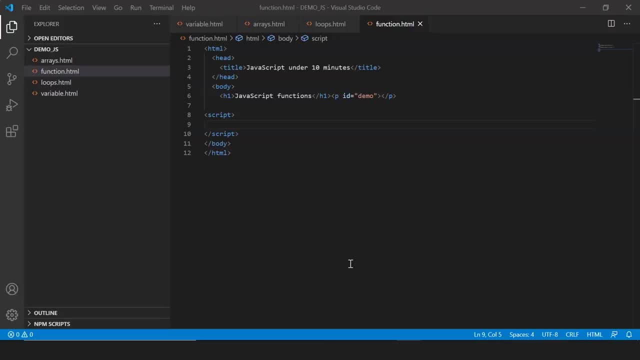 Now, when it comes to function constructor, we make use of the function keyword and the new keyword. All right, So now let's just see how it works. So let's say where my function equals new and the function keyword here, which is the. 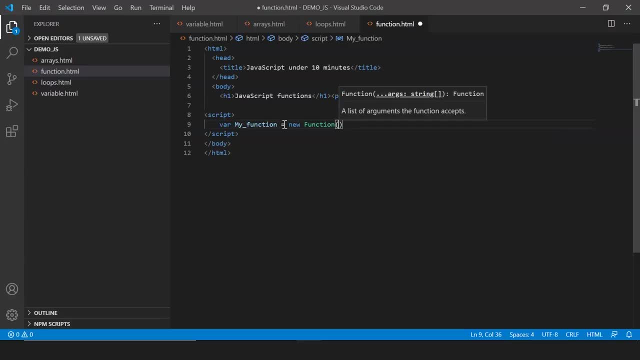 constructor, I say functionhtml. Within this I'm going to define my function. So I'm just making use of the simple sum function that adds two numbers. So let's say A and B. These two are the parameters, And when I'm returning it I say return A plus B. All right, 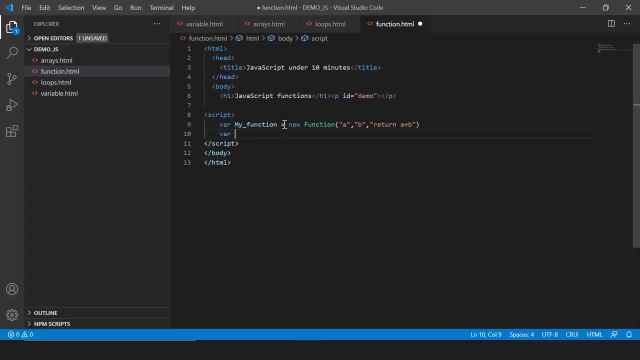 First let me define the variables. So now, when I call function, I say variable X equals my function, And I'm going to pass the digits. let's say two comma three, All right. And now let's say let. and now let's display it. 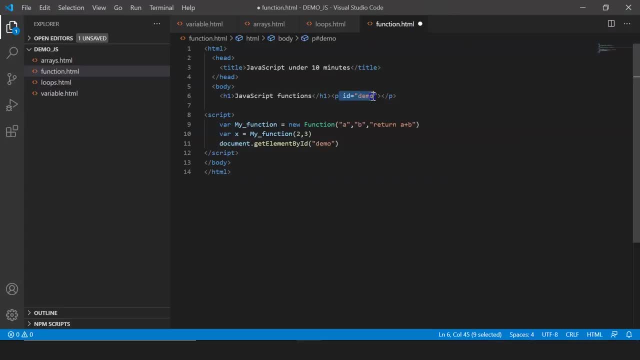 So demo. if you've seen, I've created an ID called demo here, so I can make use of that here and I say dot inner HTML: The sum is X. All right, So now let's save it and have a look at the browser. 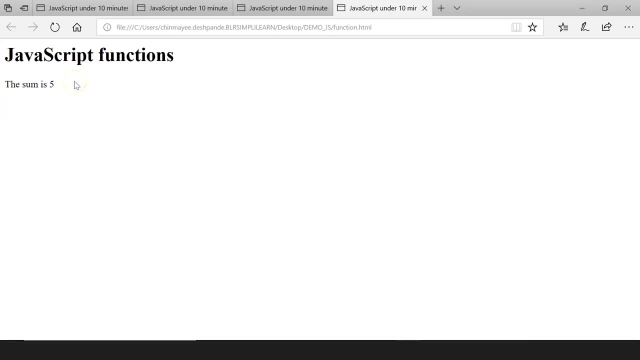 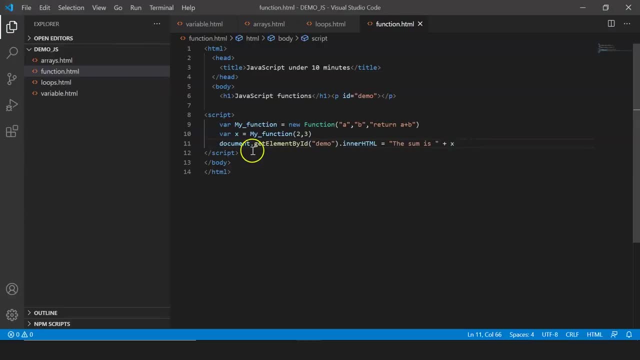 All right, So you can see, the sum five is being displayed. So now let me show you how to create a function using function expressions. So let me create another script tag, All right. And now let me say: variable Y equals function And the parameters that I'm going to be passing are A, comma, B, And when I'm defining the function,